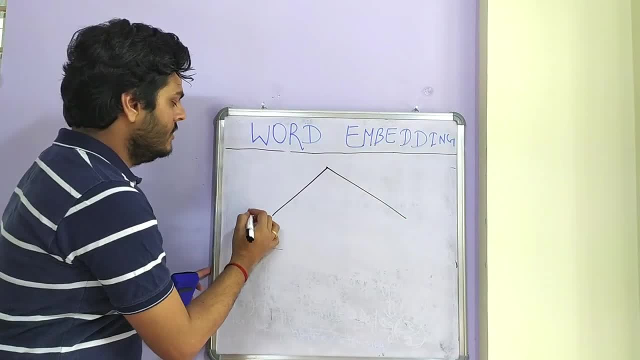 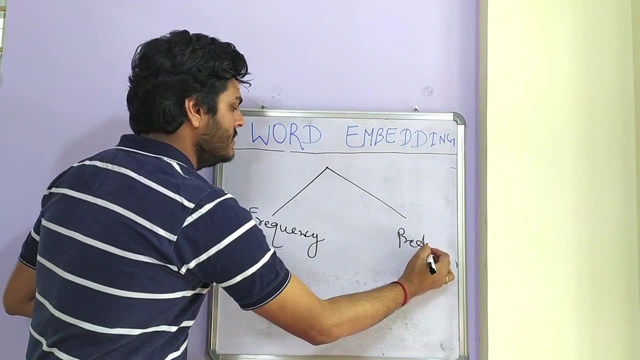 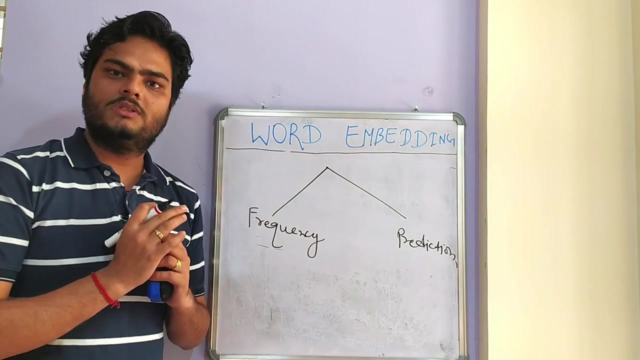 So there are basically two types of word embedding. One type is called frequency based and other type is called prediction based. In frequency based I had already covered couple of concepts. If you remember the link for the video you can see here I had covered something. 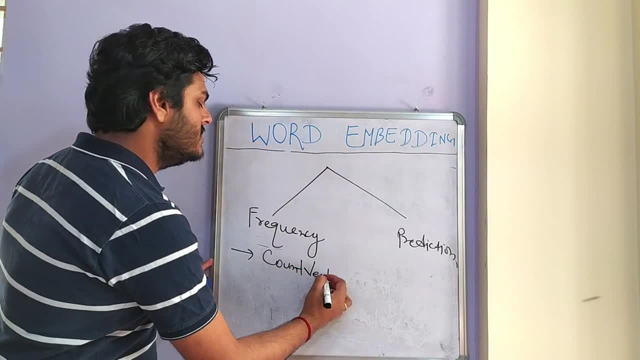 called count vectorizer, where you count the frequency of word in a document. and I had covered something called tms, So I had covered something called tms, So I had covered something called tms. So in this particular case I have covered 5 tms squared, which is 5 times the frequency. 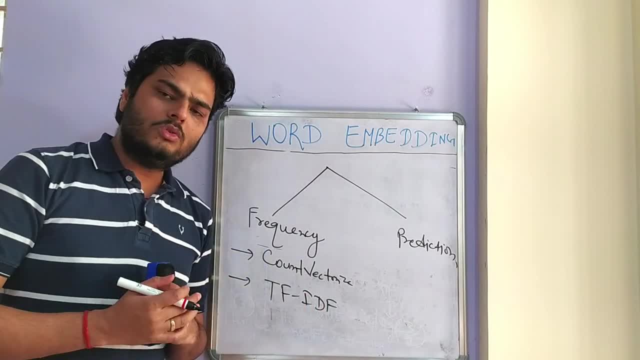 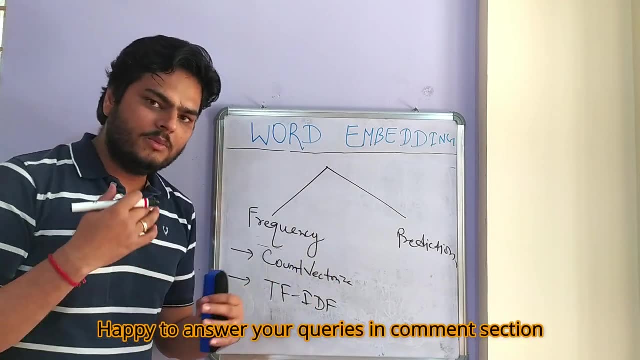 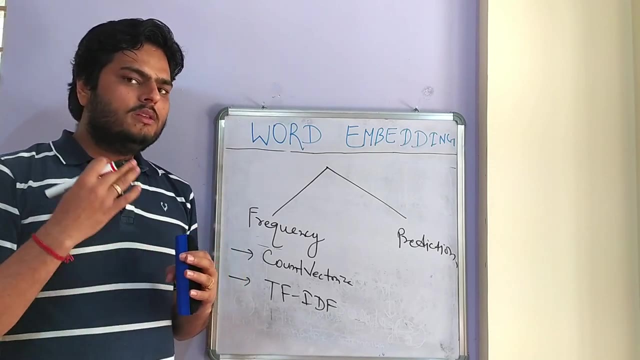 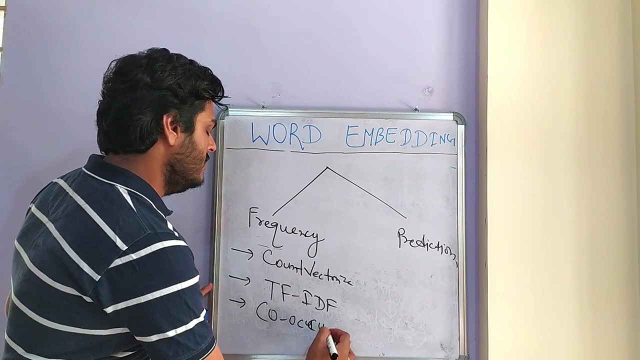 of IDF term frequency and inverse document frequency. Now, these two kinds of concepts are very important if you want a frequency based approach, because in both these implementation we use the number of times a particular word occurs in a document. There is something else in frequency based approach. This is known as co-occurrence matrix. Co-occurrence matrix. 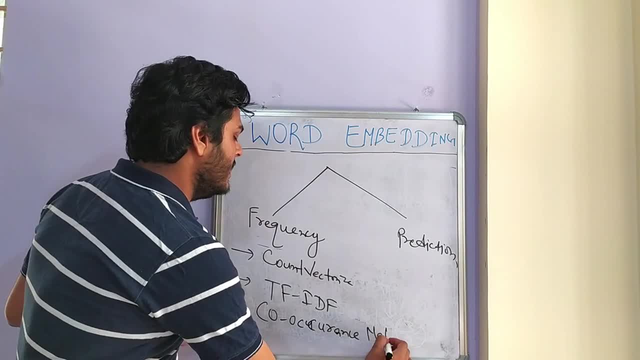 I will just explain you the name of the code. The citations you will find yourself using is the corresponding ones and based upon that set of citations you can calculate the numbers that are Nuevo Ba Jaye and Felicianoae and curve number R and patron number K. Tyler's matrics. 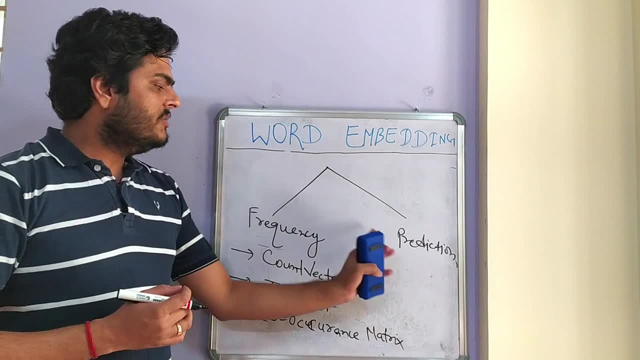 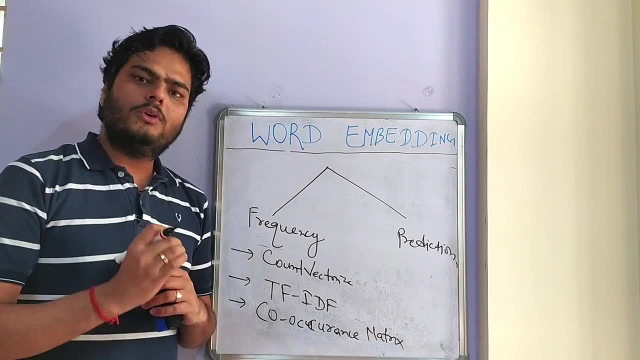 Let us see what is the the Law of juego of argument and the options The Luo's matrix requires you. what is co-occurrence matrix? in a minute before that, what is prediction based approach? so in all these approaches, we use the count of a word occurring in a document. okay, but in prediction. 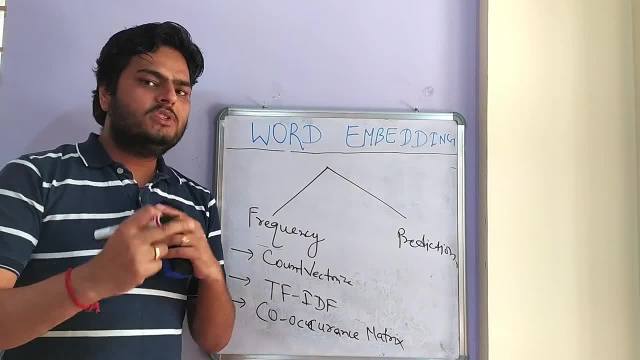 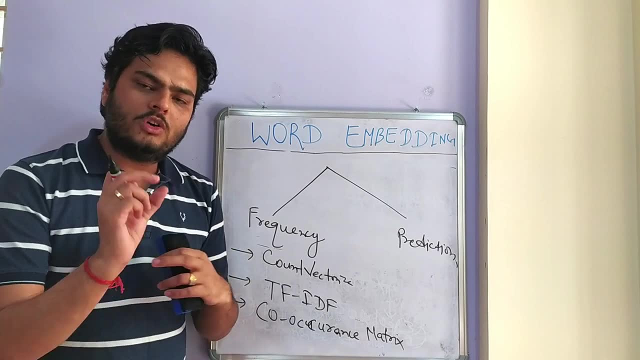 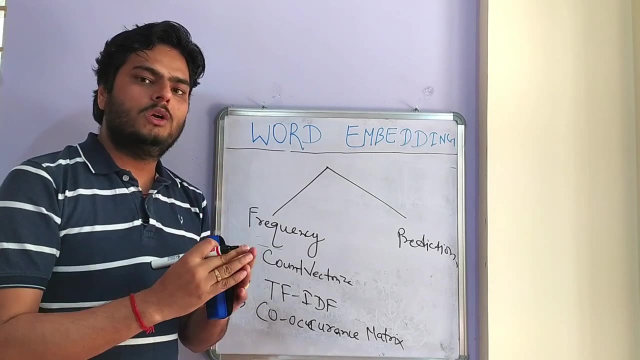 based approach. what we do is we try to capture the meaning- or i was giving the example of those two sentences in the beginning- we try to capture the context of a word in which it is used. okay, so what we do is we try to predict, based on the previous word, what would be the next word. 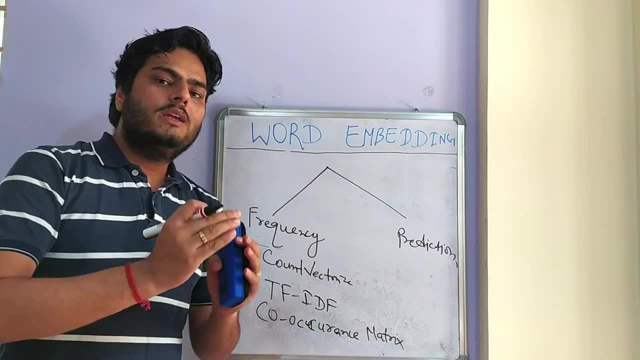 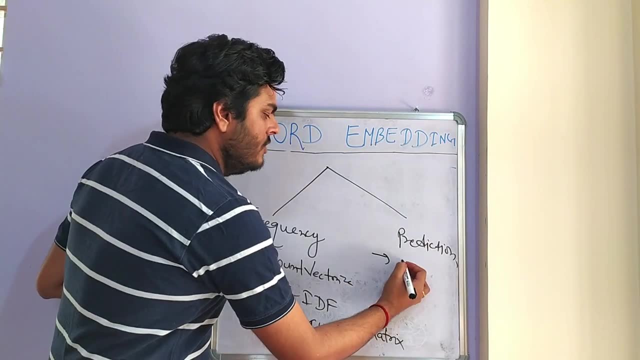 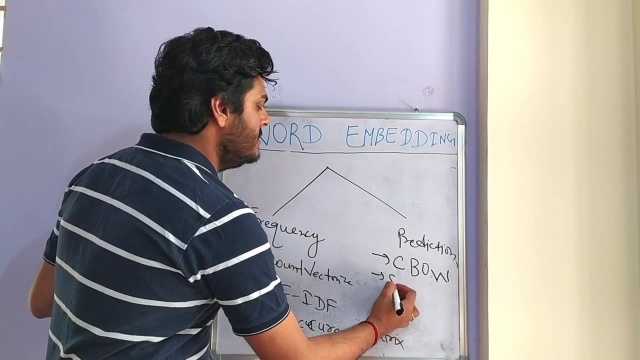 or based on the previous word. what is the nearest word to this word in this entire document? there are two concepts on which prediction based word embedding is implemented. one is known as continuous bag of words and other is known as skip gram. okay, skip gram. so on these two techniques. 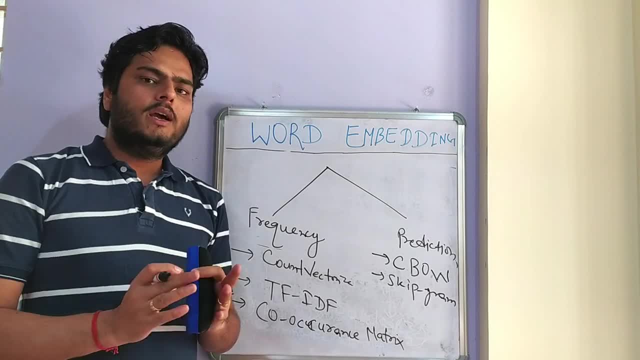 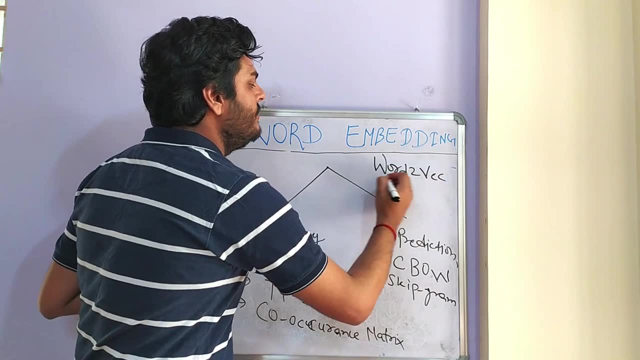 prediction based approach. we use the count of a word occurring in a minute before that. what we do is prediction based word embedding work okay, and you would have definitely heard of something called word to wake. so what to wake is nothing but a implementation by google using these techniques. 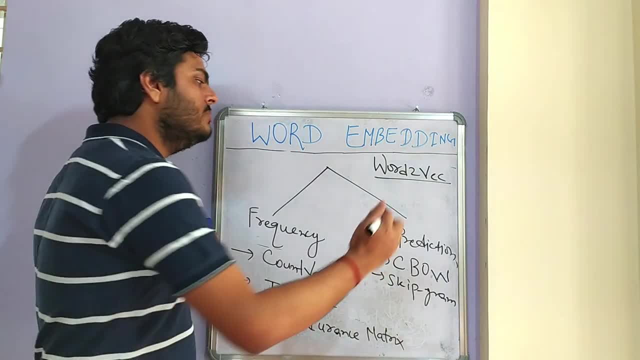 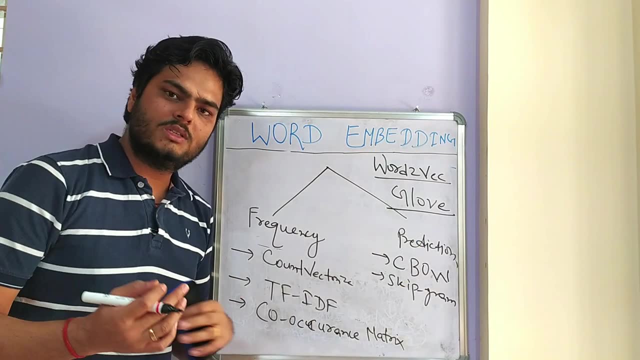 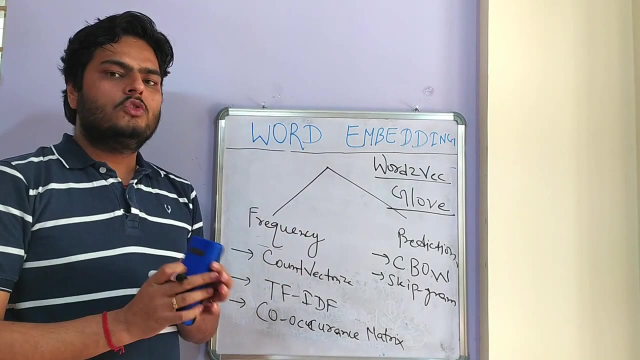 of word embedding: okay, and there is one more implementation, known as glove. you would have seen or heard this as well on some portals. so globe is nothing but another implementation of word embedding using co-occurrence matrix. okay, so what is co-occurrence matrix at first place? so this, what you see here, is nothing but a. 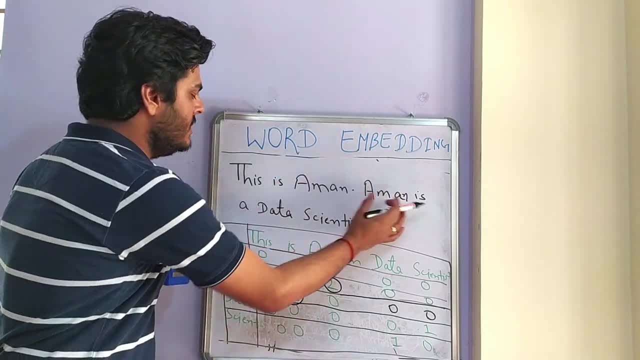 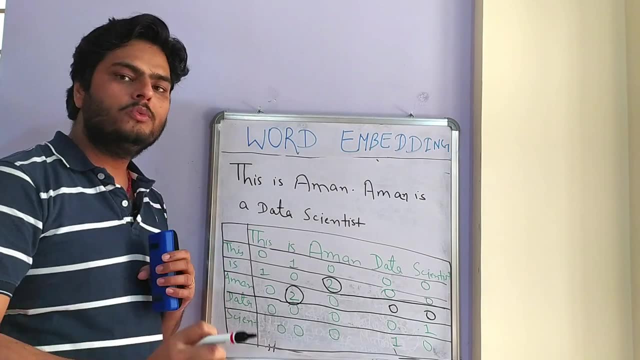 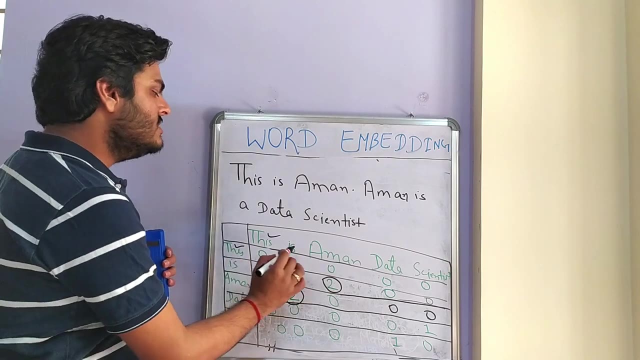 co-occurrence matrix. we have a sentence: this is aman. aman is a data scientist, the funda. here is: what is the co-occurrence of each word with each other. for example, how many times this occurs with this: zero times. how many times this occurs with is one time. how many times this occurs with aman: zero times. 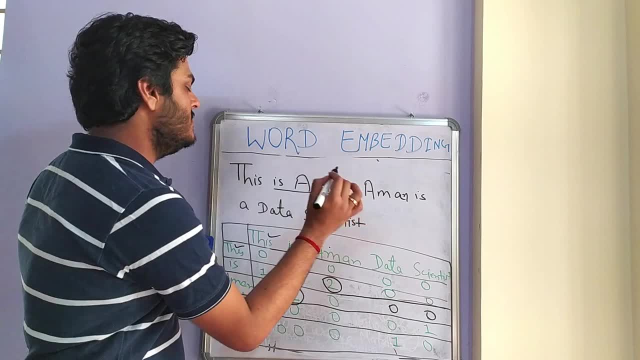 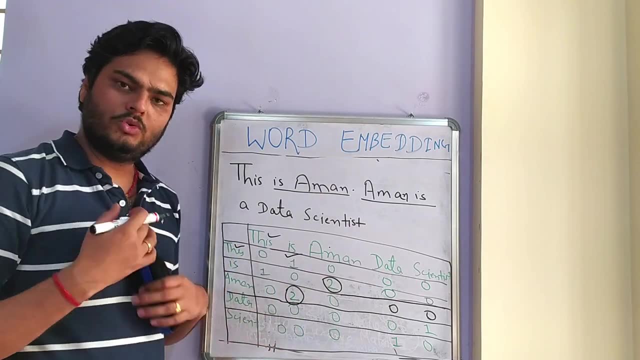 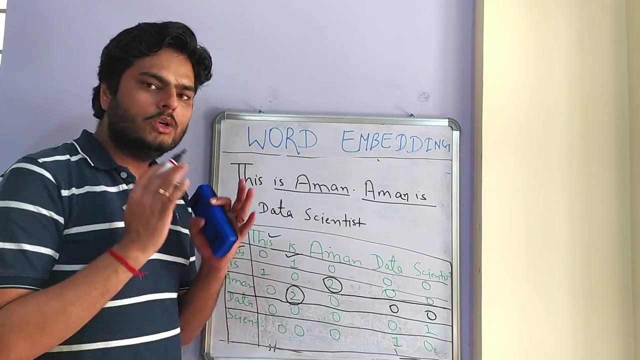 how many times is occurs with aman. so is aman is here and aman is is here. okay, hence, as aman will become two and aman is is also become two, it is just co-occurrence of the words. okay. this is known as a co-occurrence matrix. this co-occurrence matrix goes as input to the globe implementation. 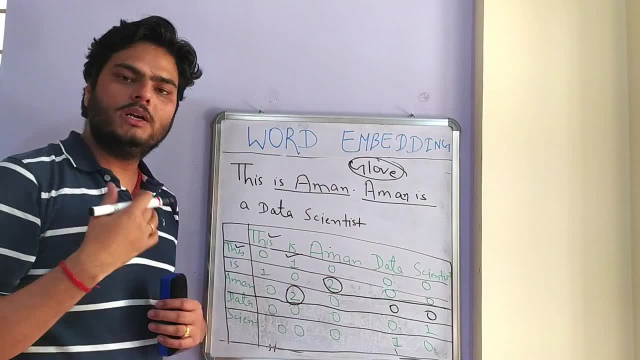 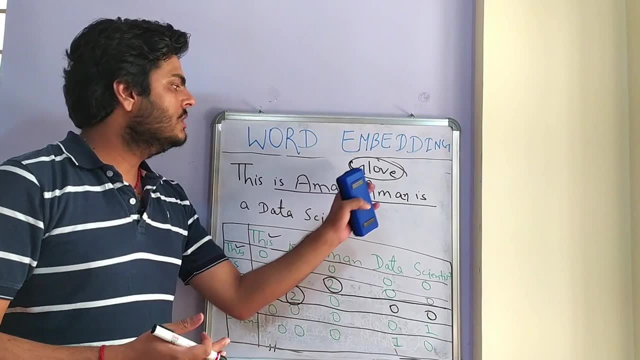 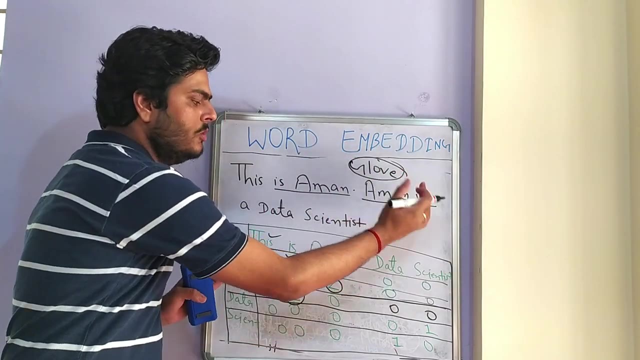 okay. so we saw two implementation of word embeddings. one is globe and other is other is what to work. so this co-occurrence matrix goes as the input to globe learning. okay, so i will explain you in detail how the word embedding is learnt in globe using co-occurrence matrix in a separate. 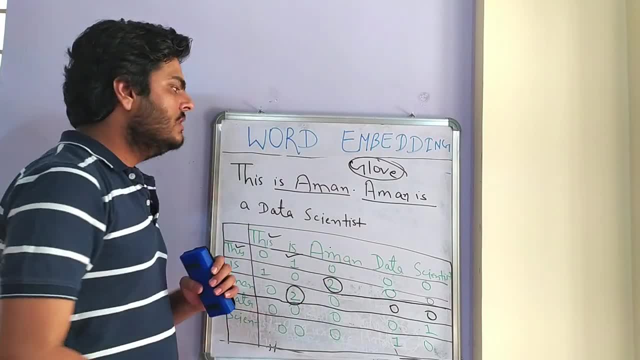 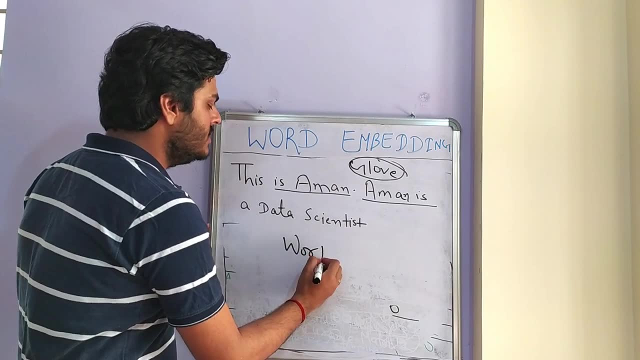 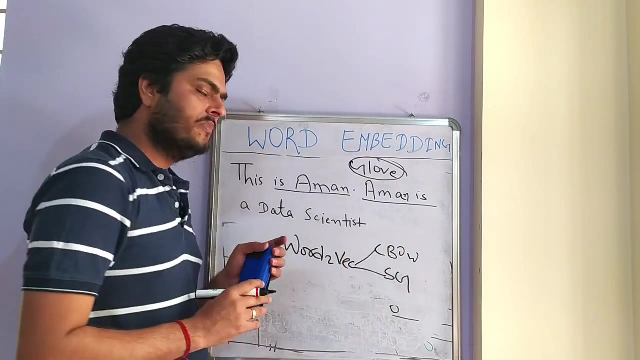 video. that is a very long topic, okay. after that, for understanding something called what to work, as i told you, what to work, implement is two things internally, okay. one is called cbow- continuous bag of words. another is called skip gram. for understanding cbow and skip gram, what you need to understand is something called neural. 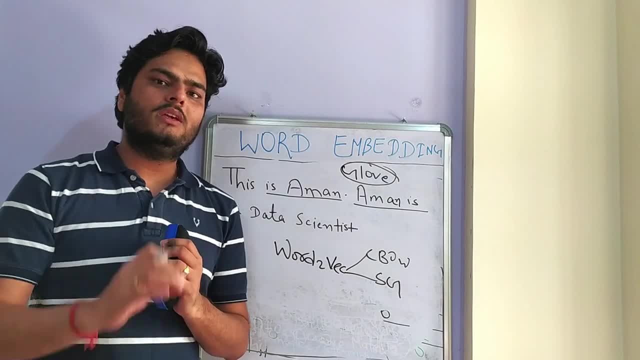 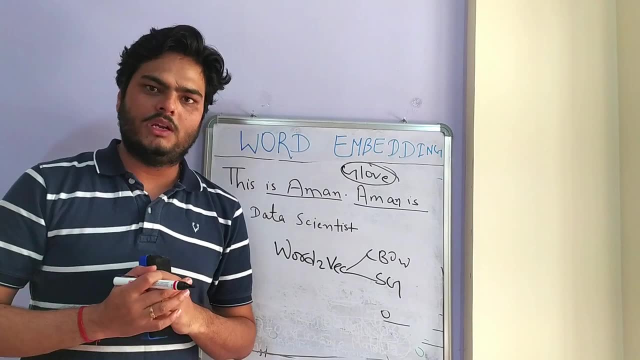 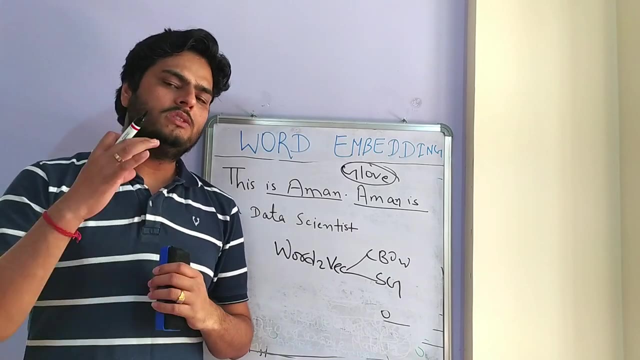 networks. so before i make you understand the inner mathematics of how these two algorithms are implemented, i want you to understand the basics of neural network. so i will create a complete set of videos on basics of neural network for understanding the basics of neural network, and we will be able to talk about this in detail. one of the following. things first, like what is a?